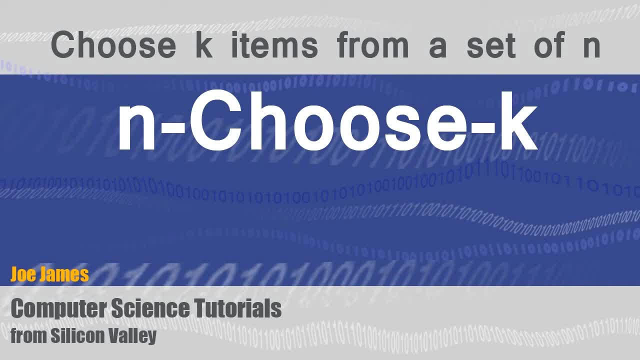 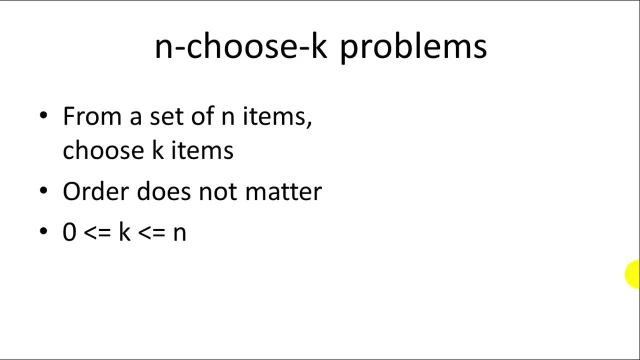 Hi, I'm Joe James and in this video I'm going to explain n-choose-k problems. This is relevant to both computer science and statistics. The problem is: from a set of n items, we want to choose k items and we're trying to determine the number of possible combinations of items. 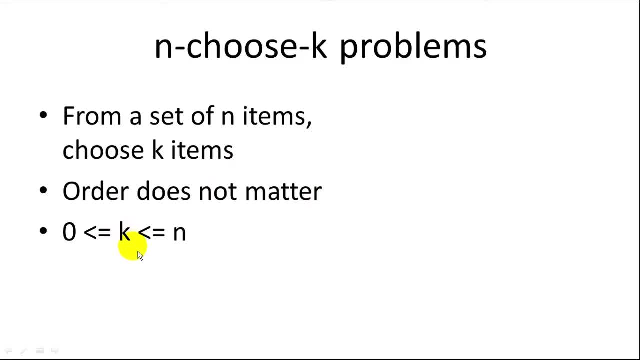 An order does not matter and the number of items we're choosing k is always going to be between 0 and n. You'll see these types of notation commonly used for n-choose-k problems. I'm going to use the upper two in this video. 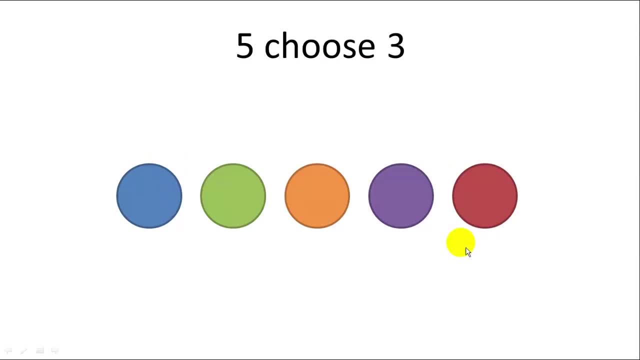 So in a five-choose-three problem, you might have five different circles and you need to choose three of those. We don't care about order, you just have to choose three, and we want to find out how many different possible color combinations there are. 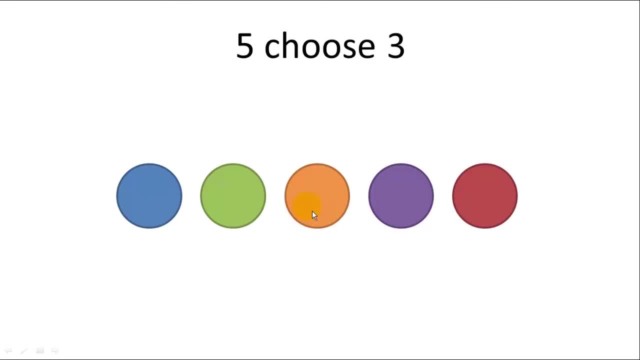 So blue, green, orange, orange, purple, red, those are two different possible combinations. That is a common n-choose-k problem. So there's a standard formula. Actually there are a couple of different ones. I'll show you here. 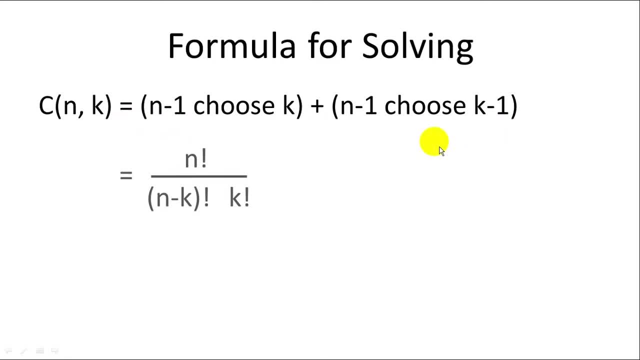 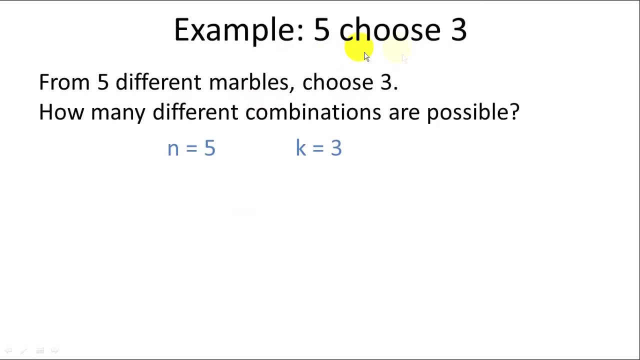 This one I'm going to explain in the next slide. The basic formula is this. So if you get one thing out of this video, remember this formula: n factorial over n minus k factorial times k factorial. So back to our five-choose-three problem. 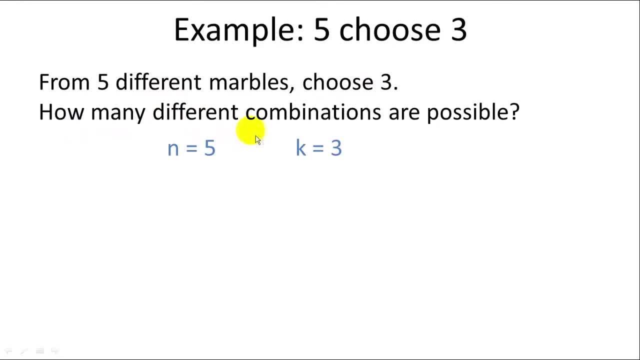 From five different marbles, choose three. How many different combinations are there? So n equals five here, because there are five different possible combinations, And k equals three because we need to choose three. So our formula is this. We're going to plug in: n equals five and k equals three. 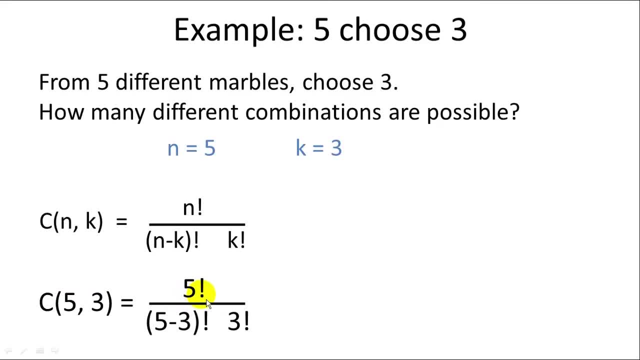 And we get the number of possible combinations is five factorial over five minus three factorial times three factorial. And five factorial is equal to five times four times three times two. Five minus three is two. So two factorial is just two And three factorial is three times two. 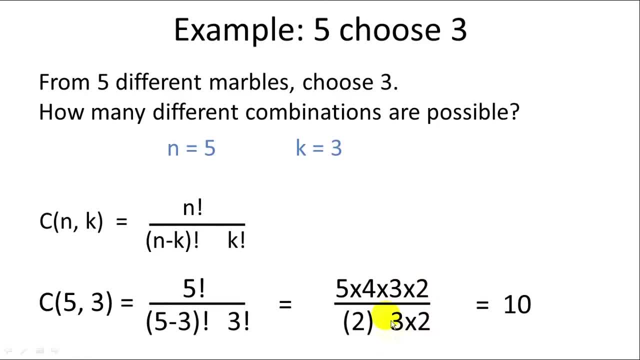 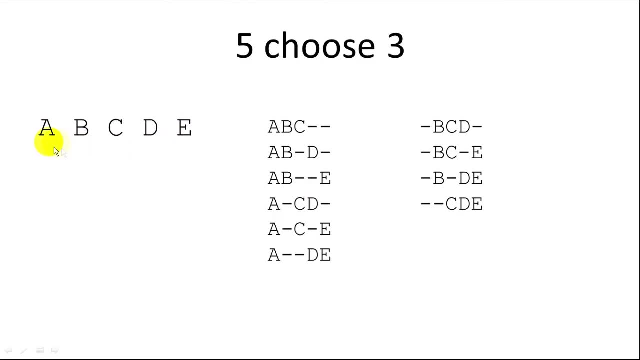 So when we work out the math we can see three times two. cancel each other out. We get five times four over two, which is ten. So there are ten different possible combinations for the five-choose-three problem. So if we were going to choose letters instead of marbles or colors, a, b, c, d, e, five-choose-three. 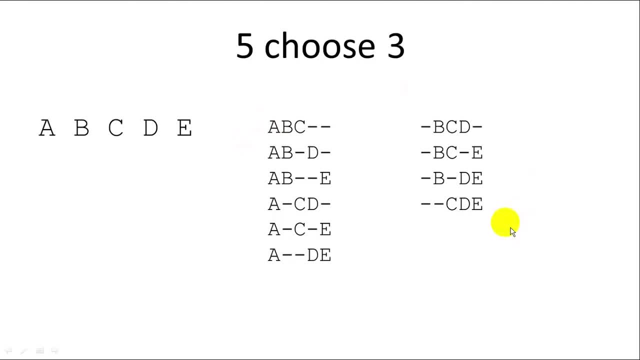 we can see the ten different possible combinations here on the right, But we could actually boil this problem down. We could reduce this problem to two smaller problems. So if we choose a, then we would need to choose two of the remaining four items. 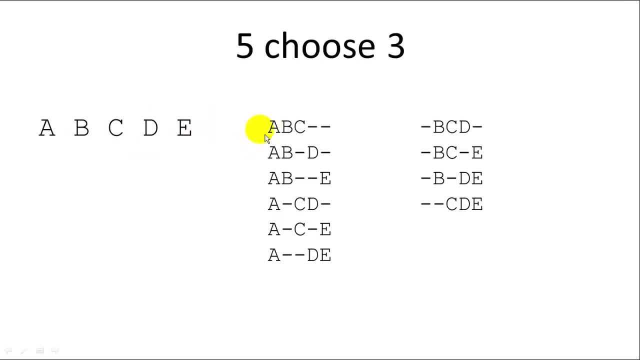 So it would become a four-choose-two problem And that's what we have here on these items on the left, You can see that we chose a for all of these And we need to choose two of the remaining four, And there are six different possibilities. 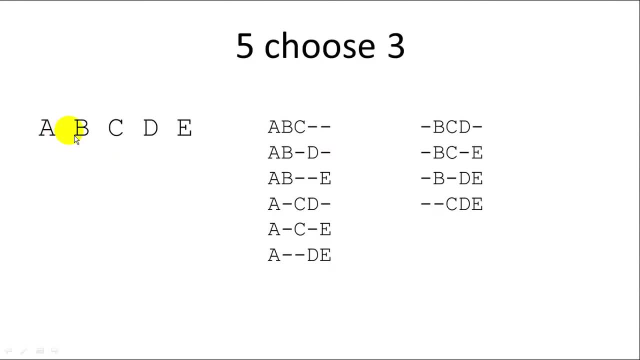 And if we don't choose a, then we need to choose two of the remaining four, And there are six different possibilities- And if we don't choose a, then we need to pick three of the remaining four items, which is what we have here on the right. 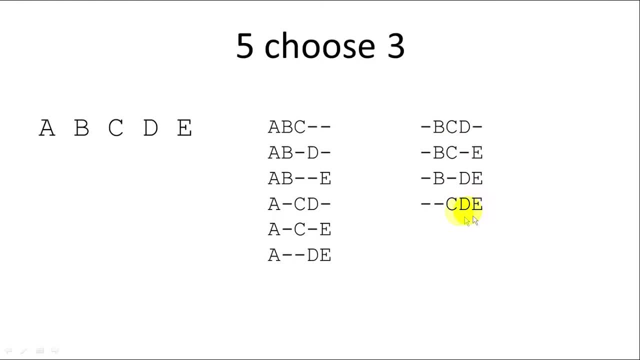 We have a not selected and we have to choose three of the remaining four items, And we can see there are four different combinations. So the n-choose-k problem can be reduced to n minus one- choose k minus one. plus n minus one- choose k, which is exactly what we've done here in this. 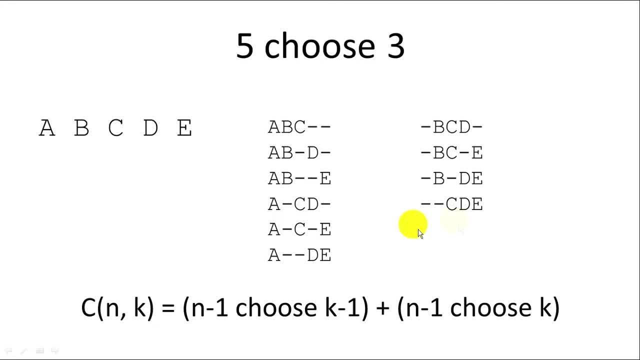 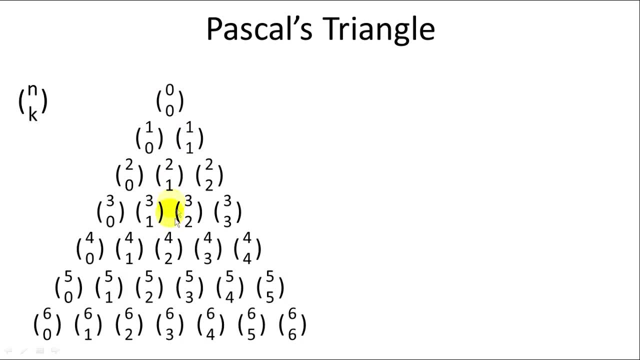 And that suggests that n-choose-k problems could be solved recursively in computer programming. Another way to look at n-choose-k problems is using Pascal's triangle. When we structure a triangle like this, with n on top and k on the bottom, and the top number is the row number, so we can see row number zero, row number one, row number two, row number three. 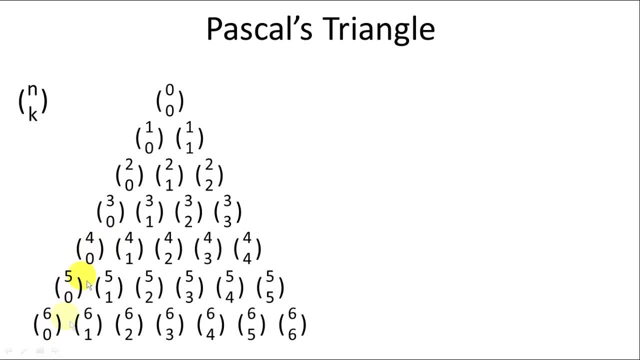 And k basically starts from zero at the left item and increases by one each item to the right. And k basically starts from zero at the left item and increases by one each item to the right. And k basically starts from zero at the left item and increases by one each item to the right. 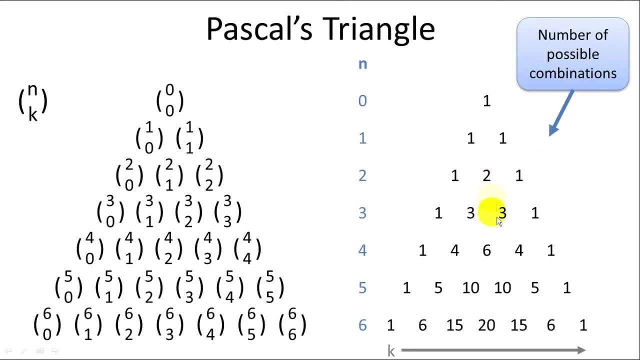 So what Pascal found is that the number of combinations possible when you structure a triangle like this- for, let's say, this cell here, which would correspond to four, choose two- is equal to the sum of the two cells directly above it. So this three and this three added together makes six.